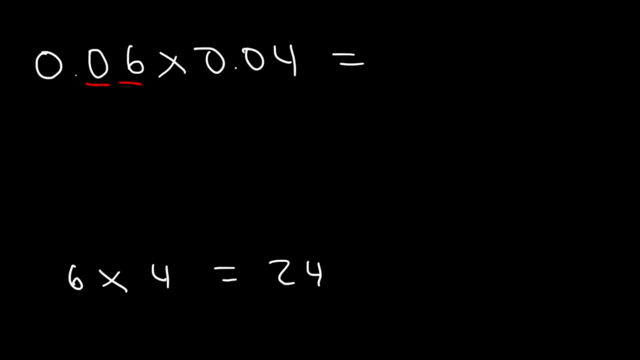 In the first number there are two digits to the right of the decimal point, and the same is true for the second number. When you're multiplying, add these two digits: 2 plus 2 is 4.. So your final answer should contain four digits after the decimal point, and you need a 2 and 4 as well. 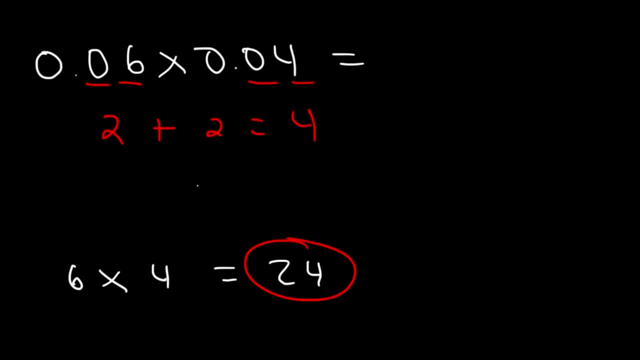 So because 6 times 4 is 24, 0.06 times 0.04 is going to be 0.0024.. You need to have a total of four digits to the right of the decimal. Now let's try another example. 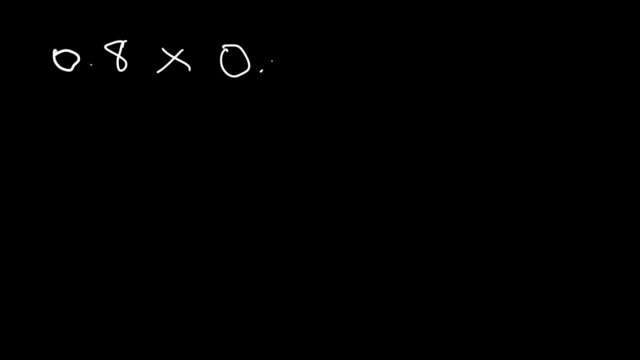 What is 0.8 multiplied 0.08, multiplied by 0.07.. Go ahead and try this one. So first we know that 8 times 7 is 56.. Now let's look at the digits that we have. 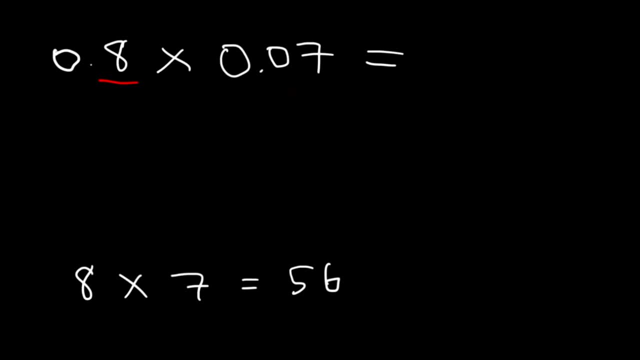 The first number has one digit to the right of the decimal point. The second number has two: 1 plus 2 is 3.. So our answer should have three digits to the right of the decimal point. So since 8 times 7 is 56, 0.8 times 0.07.. 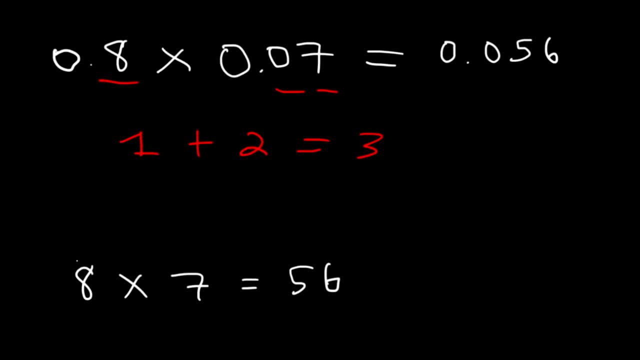 It's going to be 0.056.. And, as you can see, we have three digits to the right of the decimal point. So, based on those two examples, go ahead and try these three: Multiply 0.6 times 0.8, 0.09 times 0.07, and also 0.12 times 0.005.. 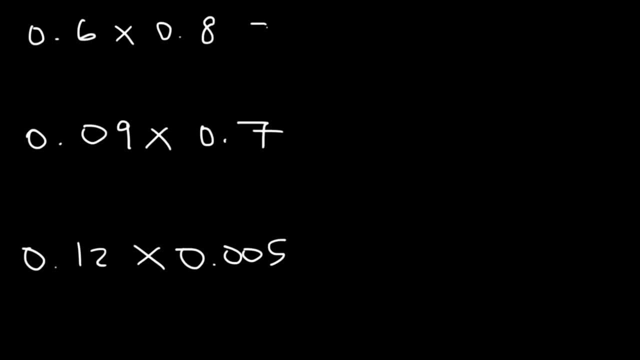 Go ahead and try these three examples. Now we know that 6 times 8 is 48.. So 0.6 times 0.8 is 0.48.. Now let's check the digits. We have one digit in the first number to the right of the decimal point, and one as well. 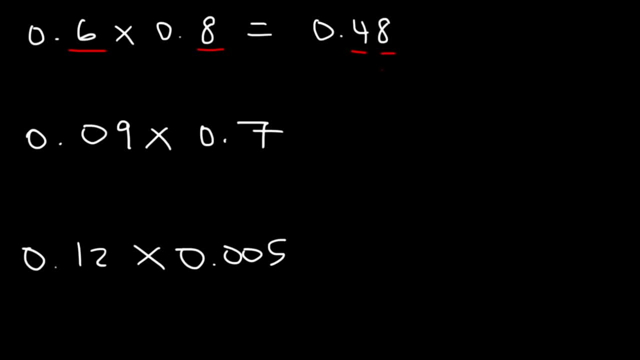 1 plus 1 is 2.. So the final answer should contain two digits. Now looking at the next number: 9 times 7 is 63.. So 0.09 times 0.07.. It turns out it's 0.063.. 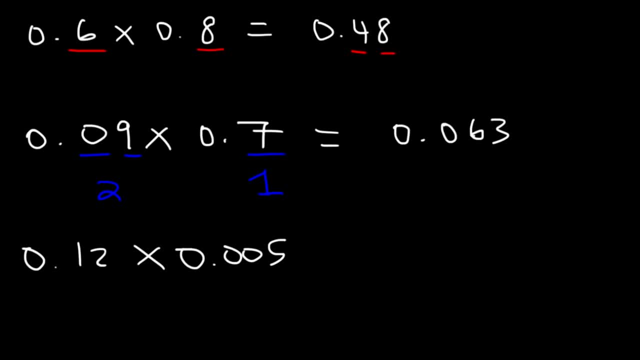 Here we have two digits, Here we have 1.. 2 plus 1 is equal to 3.. So we need a total of three digits in our answer. Now what about the last one? 12 times 5 is 60.. 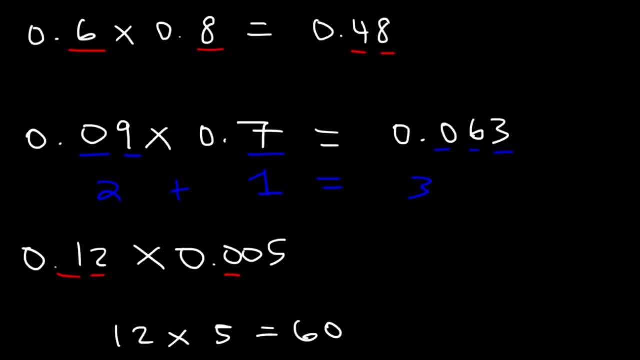 The first number has two digits. The second one has three digits. 2 plus 3 is 5.. So our answer has to contain five digits. So this is going to be 0.00060.. Make sure you have the extra 0 to the right of the 60 for this to work. 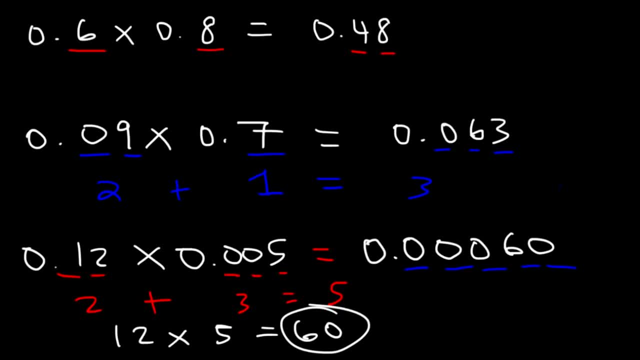 Notice that we have a total of five digits. Now, if you have a 0 at the end, you really don't need to write it, So you need to understand that this is equivalent to 0.0006.. It's the same. 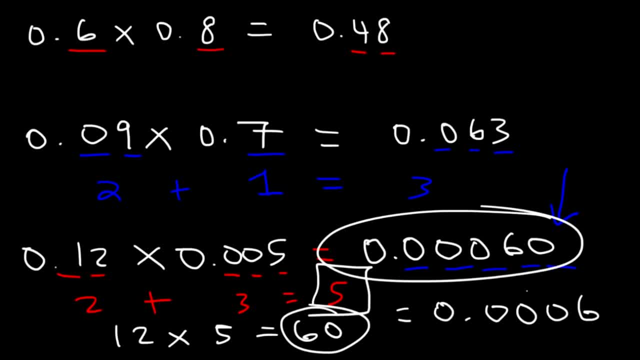 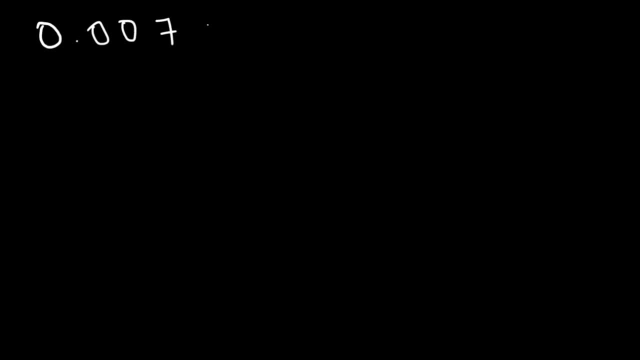 But first you want to write it this way, Using the same, And then you can just rewrite it like that. But if you type it in your calculator, your calculator is going to show this answer. Now, what about dividing two numbers? What are the rules for this situation? 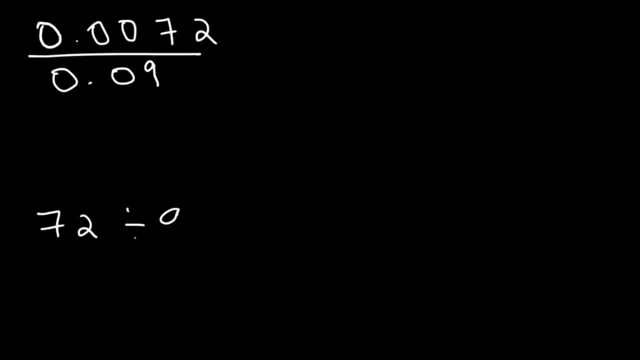 Well, we know that 72 divided by 9 is 8.. Because 8 times 9 is 72.. But what is 0.0072?? What is 0.0072 divided by 0.09?? Well, let's compare multiplication and division. 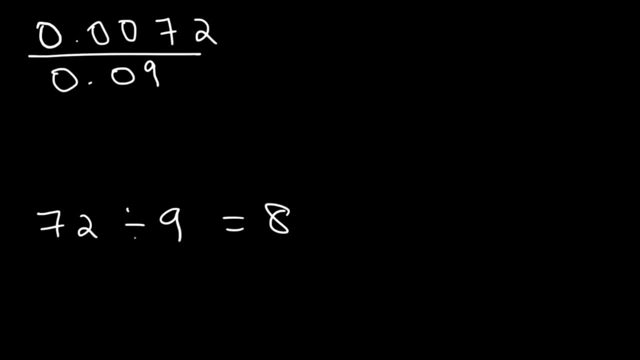 When multiplying decimal numbers, you need to add the digits. When dividing decimal numbers, you need to subtract the digits. So, looking at the top number, there's four digits And the bottom number has two. 4 minus 2 is equal to 2.. 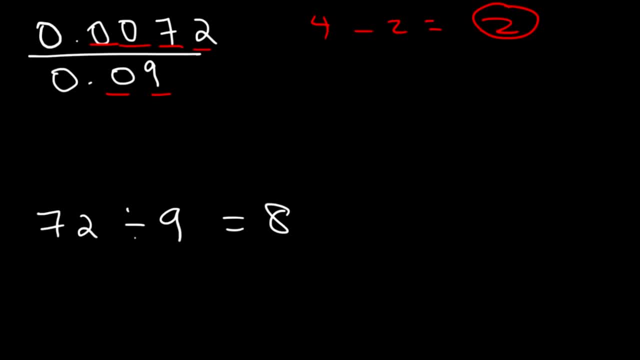 So, therefore, your final answer should contain two digits, Since 72 divided by 9 is 8, 0.0072 divided by 0.09 is going to be 0.08.. So that it has two digits to the right of the decimal. 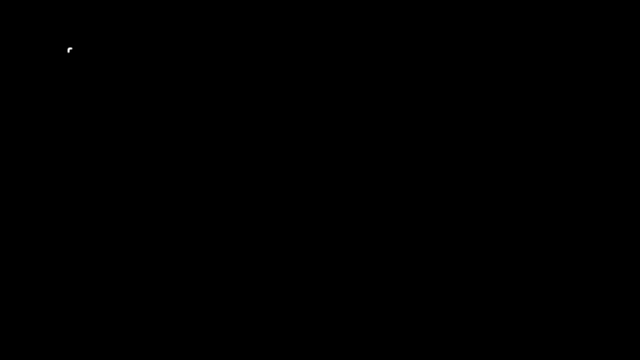 So let's try another example. Let's divide 0.054 by 0.6.. Now, 54 divided by 6. 56 is 9.. And on the top we have three digits. On the bottom we only have one. 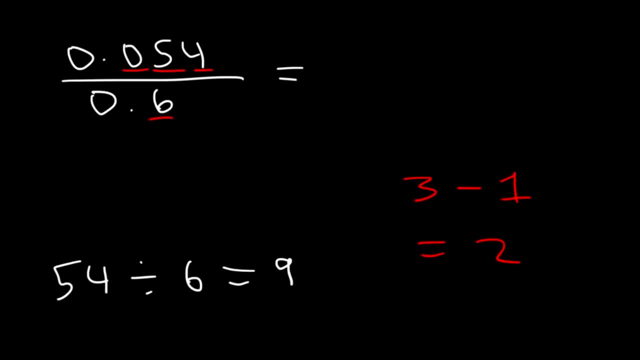 3 minus 1 is 2.. So the final answer should have two digits. So this is going to be 0.09.. So now it's your turn. Try these three. Feel free to pause the video as you work on these three examples. 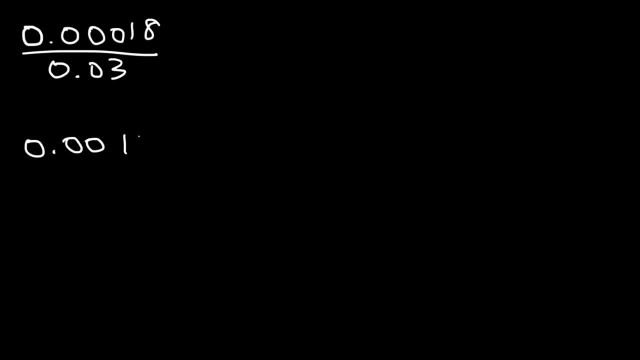 And here's the last one, So let's start with the first one. First, let's look at the digits. On top there are five digits and on the bottom there's two. Five minus two is equal to three, So the final answer should have three digits. 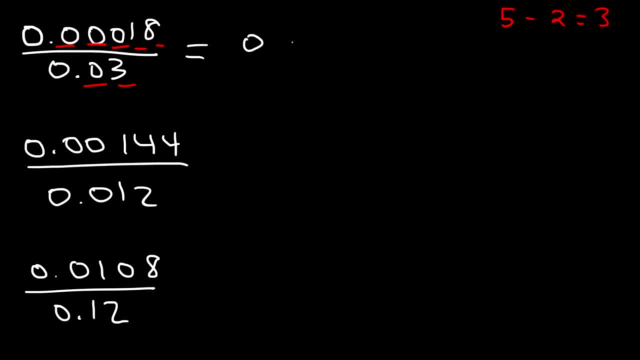 Eighteen divided by three is six. So this is going to be point zero zero six. Now, looking at the next one On top, there are also five digits. On the bottom we have three digits to the right of the decimal, And five minus three is two. 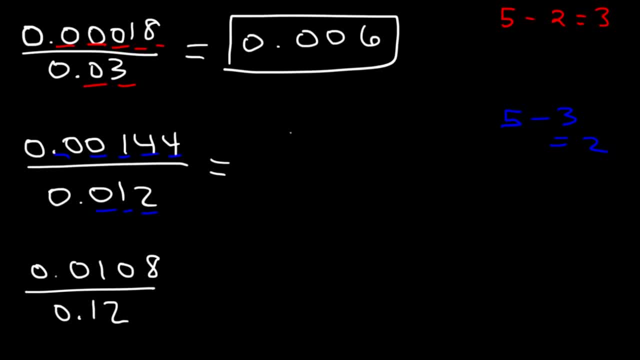 Now, one forty four divided by twelve is twelve, So to have two digits is just going to be point one, two or point twelve. Okay, And so that's the answer. And now for the last one. There are four digits on top and two on the bottom. 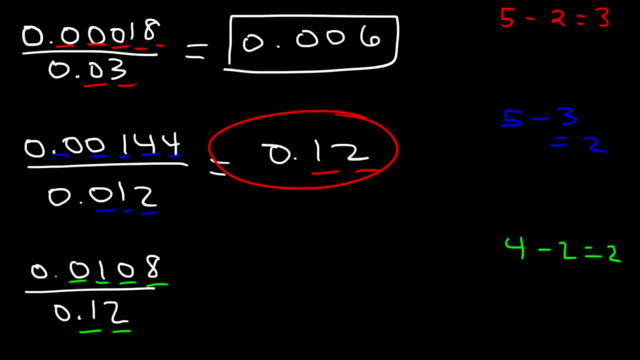 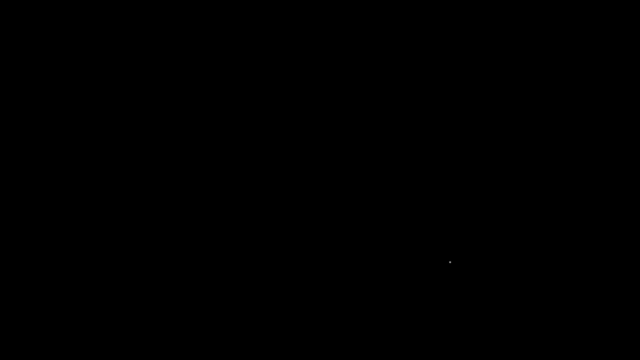 Four minus two is two, Now one. oh, eight divided by twelve is nine. So this is going to be equal to point zero nine. So that's how you can divide two decimal numbers. So far, we've considered situations in which the numerator had more digits to the bottom. 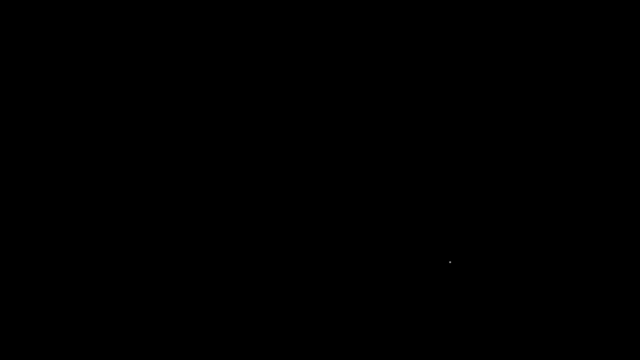 And the denominator had more digits to the right of the decimal point than the denominator. But what if they're the same? or what if the denominator has more? What's going to happen in that case? So, for example, let's divide point twelve by point zero three. 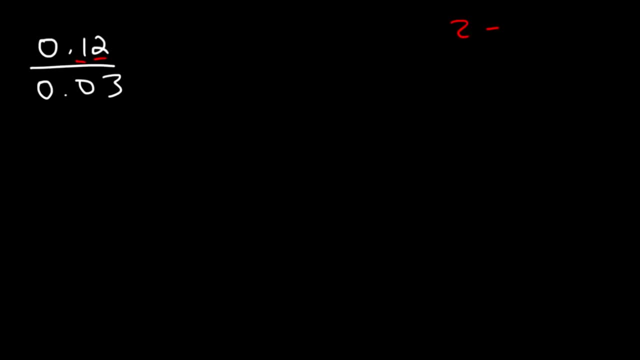 So on the top we can see that there's two digits to the right of the decimal point And on the bottom there's also two. Two minus two is zero. If you get zero or a negative number, Add one to that number. Zero plus one is one. 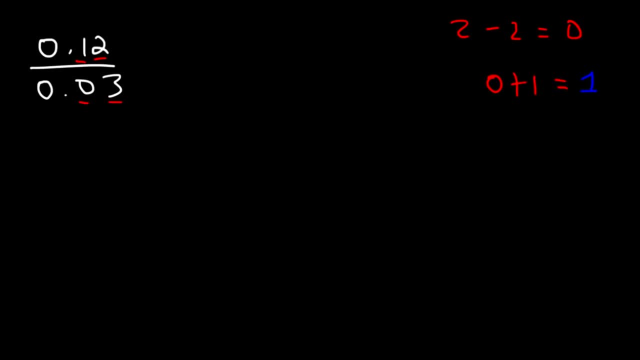 So what this means is that you're going to have one digit to the left of the decimal point. Twelve divided by three is four, So your answer is simply four. I'm going to put the decimal point here, Or four point. oh, if you want to leave it like that, 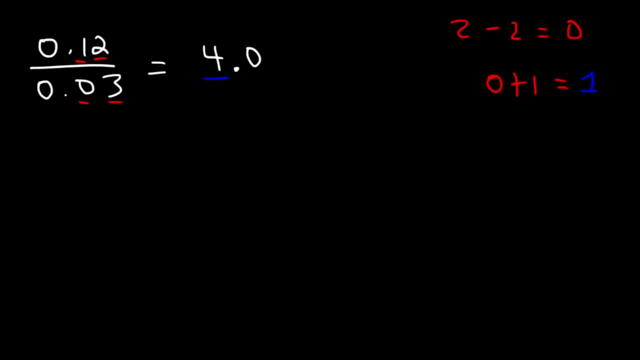 So there's one digit to the left of the decimal point. Let's try some more examples Now. let's divide point zero, Point zero eight by point zero zero two. So on top we have two digits and on the bottom we have three. 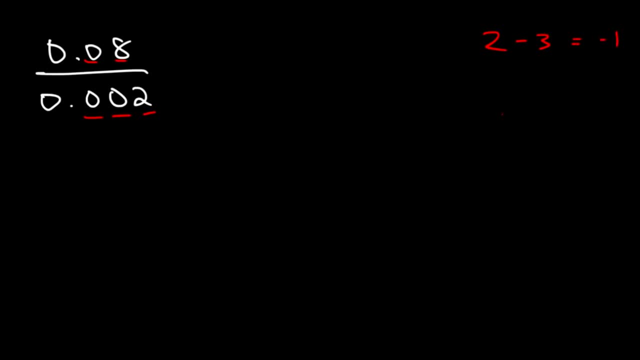 Two minus three is negative one. Now we're going to add one to negative one. However, We're not going to say Negative one plus one is zero. We're going to treat this as if it's equal to a positive one. So what we really need is the absolute value of negative one and just add one to it. 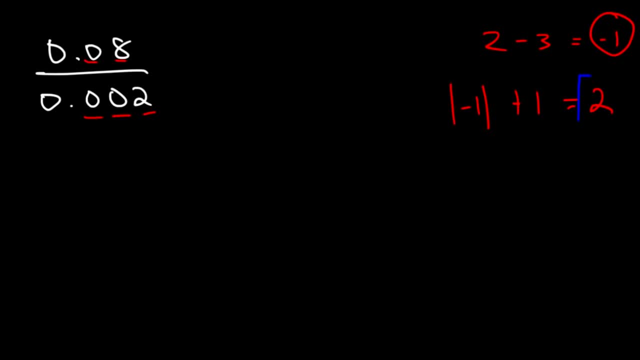 So we're going to have two digits to the left of a decimal point. If you add negative one to one, it's going to be zero, and you're not going to know what to do with that. Now, eight divided by two is four. So if we're going to have two digits to the left, 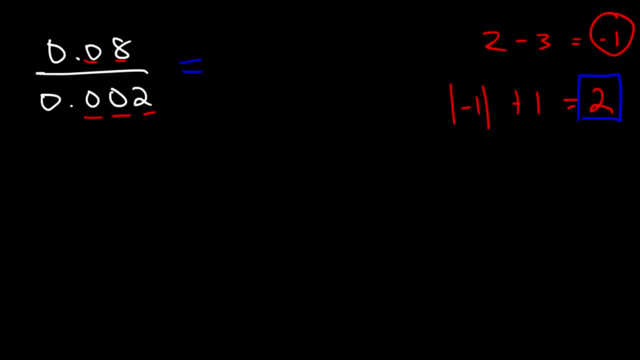 To the left of the decimal point and we need a four, then the only way to write this is forty or forty point zero. As you can see, we have two digits to the left of the decimal point and if you type this in your calculator, it's going to give you forty. 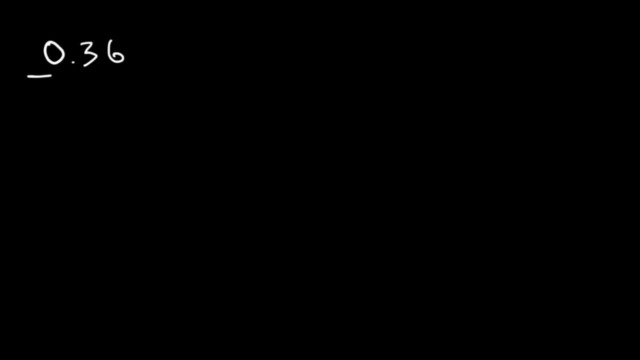 Let's try another example. Let's divide point three, six, By point zero, zero, zero, four. So there's two digits on top, As you can see, it's one, two. On the bottom, there's a total of four. So two minus four is a negative number. 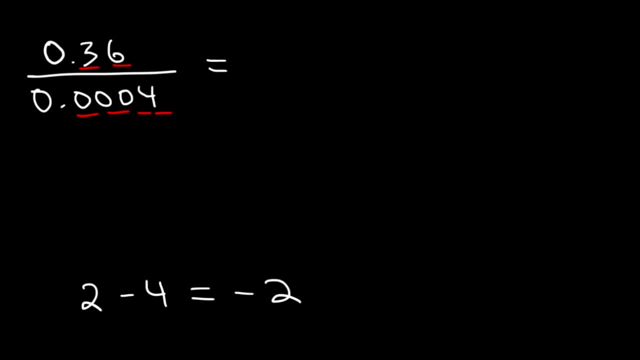 If you get zero or a negative number, make sure to add one to it, But treat negative two as if it's positive two. Then add one, Don't add one to negative two. It's not going to work. So this tells us that we should have three digits to the left of a decimal point. 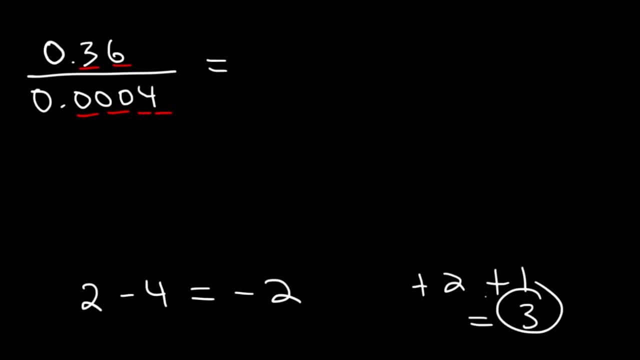 So we're going to have two digits to the left of a decimal point. So we're going to have two digits to the left of a decimal point. Let's try another example Now. thirty six divided by four is equal to nine. So how can we write a number that has a nine and that has three digits to the left of a? 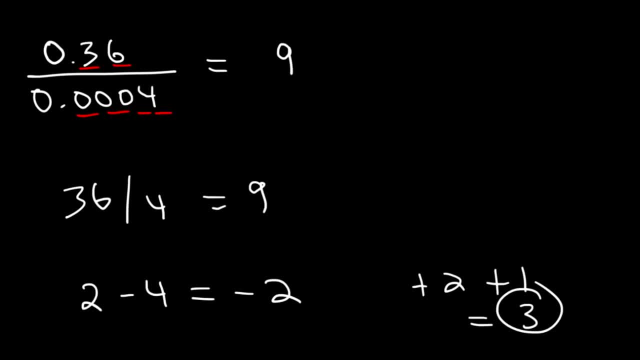 decimal point. All you need to do is add some zero's to it, So it's going to be nine zero, zero and then decimal point And, as you can see, we have three to the left Point: three, six divided by point: zero, zero, zero four is nine hundred. 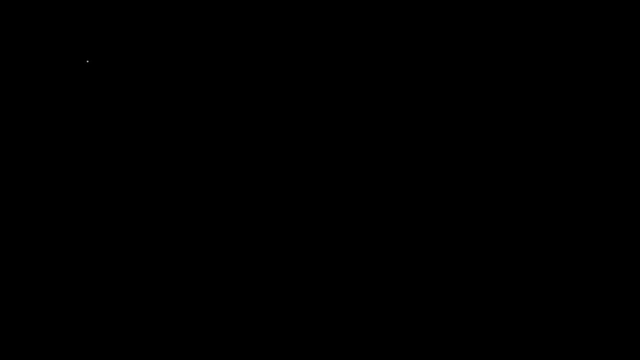 So last example on this plan, this type of problem. So let's say, if we have 0.042 divided by 0.000014.. Go ahead and try this example. So in the numerator of the fraction we have 3 digits and in the denominator there. 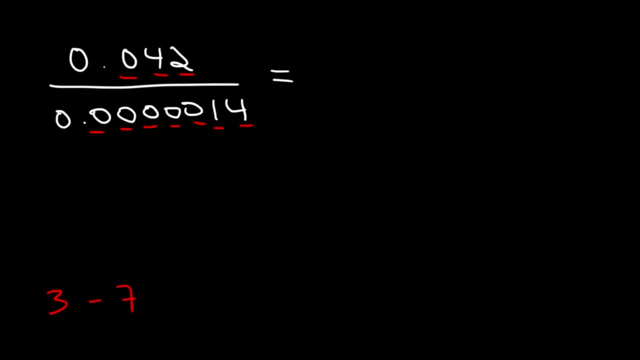 are 7 digits. 3 minus 7 is negative 4, but let's treat it as if it's a positive 4 and then add 1.. So that's 5.. Now, 42 divided by 14, that's equal to 3.. So we need 5 digits. 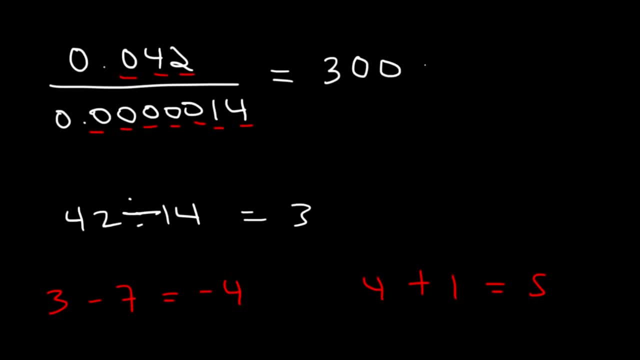 to the left of the decimal. So that's a 3 with 4 zeros, giving us a total of 5 digits on the left. So this is going to be 30,000.. And if you type it in your calculator, 0.042 divided by 0.000014 is indeed 30,000.. 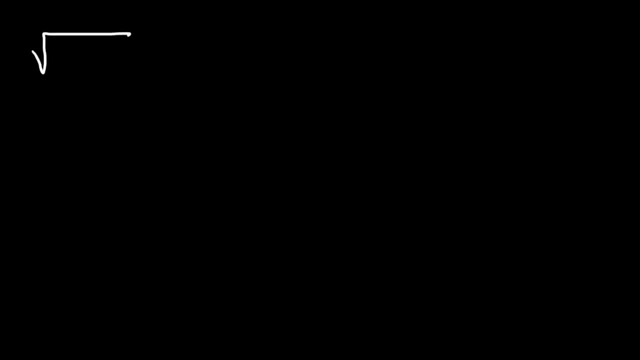 Now what about taking the square root of a decimal number? Let's say, if we want to find the square root of 0.04.. What rules can we employ to make this easier? How can we find the answer easily? So first, what is the square root of 4?? The square root of 4 is 2, because 2 times 2 is. 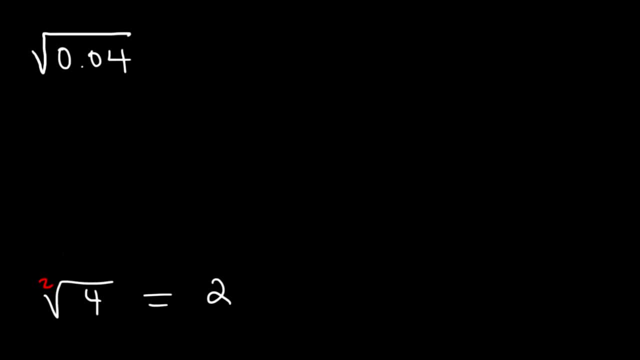 4.. The index number of the square root is a 2. If you don't see a number, it's always assumed to be a 2.. Now here's what you need to do: Count the number of digits that are to the right of 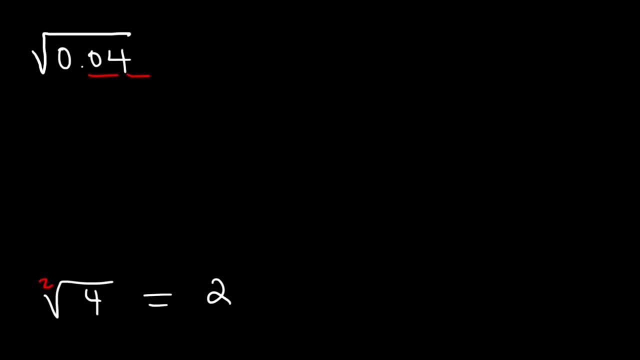 the decimal point. So notice that we have 2 digits And what we're going to do is take the number of digits and divide it by the index number. So 2 divided by 2 is 1.. Now when you divide it, you need to make sure. 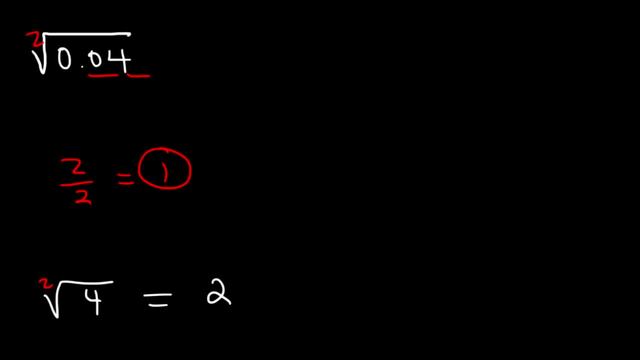 that you get a whole number. If you get like a decimal, it's not going to work. So divide the number of digits that you have by 2, and your final answer should contain this: many digits. So 0.04 has 2 digits. so the square root of 0.04 is going to be 0.2.. So notice that it. 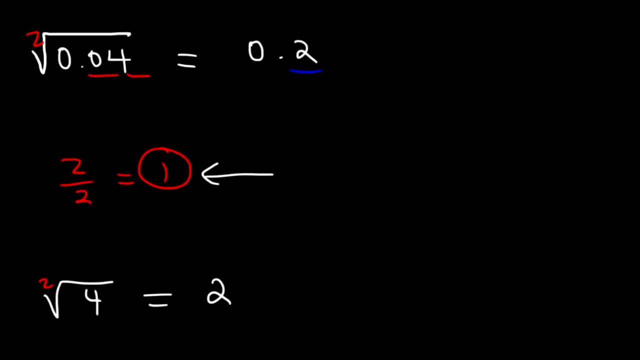 only has 1 digit to the right of the decimal point. Let's try this one: 0.0025.. Now we know that the square root of 25 is 5. And it's a total of 4 digits to the right. So 4 divided by 2 is 2.. So when you multiply decimals, you 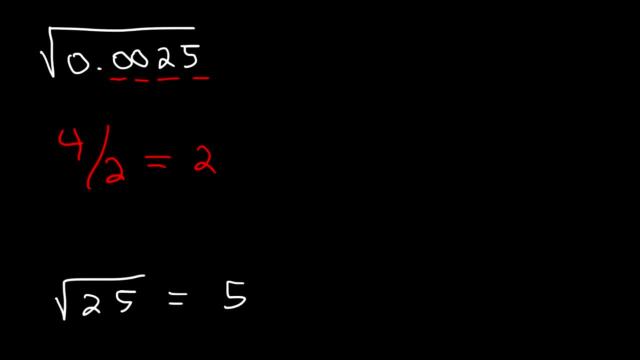 need to add the digits. When you're dividing, you need to subtract the digits. When you're multiplying by the square root, you need to divide the digits. So our final answer should have 2 digits to the right of the decimal point. So this answer. 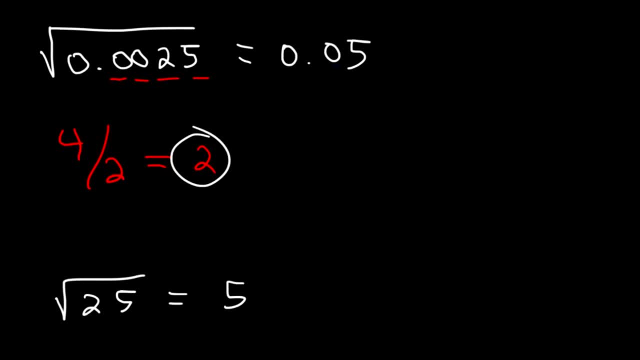 is 0.05.. Try these two: The square root of 0.36 and the square root of 0.0049.. So 0.36 contained 2 digits, and 2 divided by 2 is 1.. So the final answer should have 1 digit to the right. 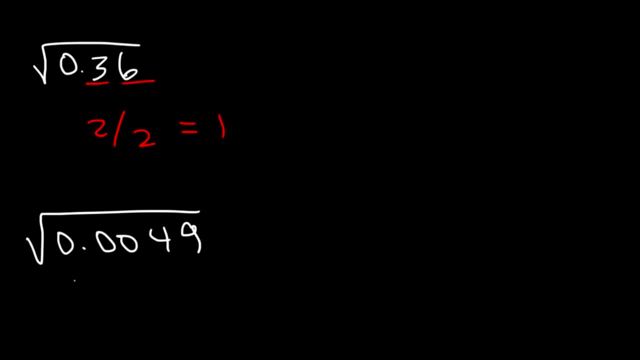 of the decimal point Now, the square root of 0.36, well, the square root of 36, let's do that first. that's equal to 6.. So the square root of 0.36 is going to be 0.6,, since this contains only 1 digit. 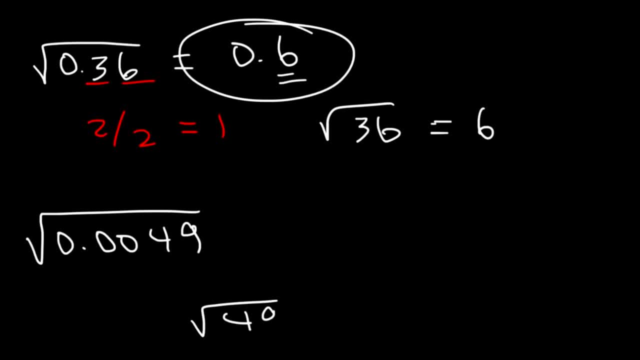 to the right Now. the square root of 49 is 7. And this number has 4 digits. So 4 divided by 2 is 2.. So the final answer has to contain 2 digits, So this is going to be 0.07.. 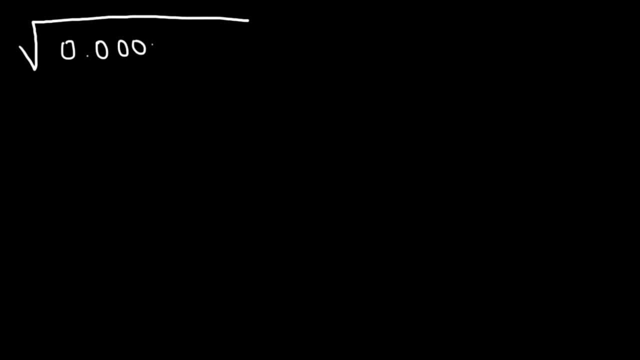 Go ahead and try these two: The square root of 0.00064.. And also, let's try a much longer one: 0.000000.. 0.000000., 0.000000.. 0.000000000.. 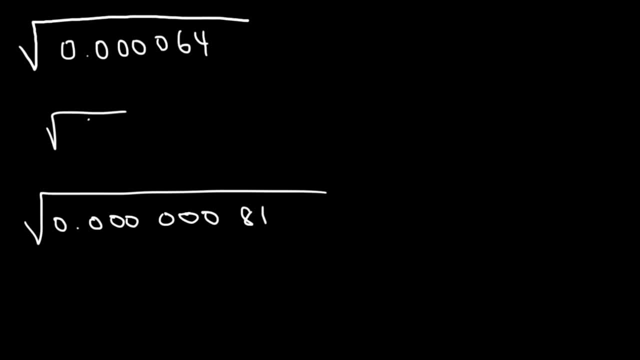 0.000000000811.. The square root of 64 is equal to 8.. And here we have a total of 6 digits. 6 divided by 2 is 3.. So the answer has to contain 3 digits to the right of the decimal point. 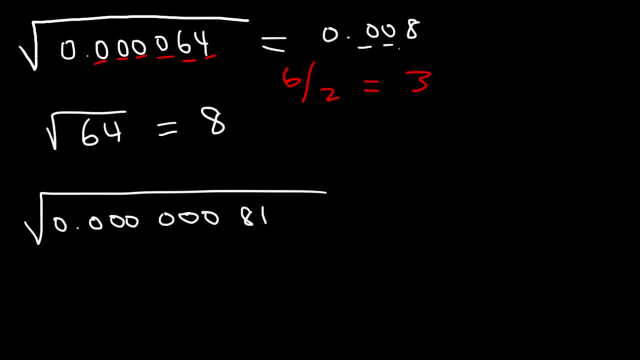 So its going to be 0.008.. Just add 2 zeros and the 8.. Now, in the next number, We have a total of 8 digits, and if we divide it by 2, our answer should contain 4 digits. 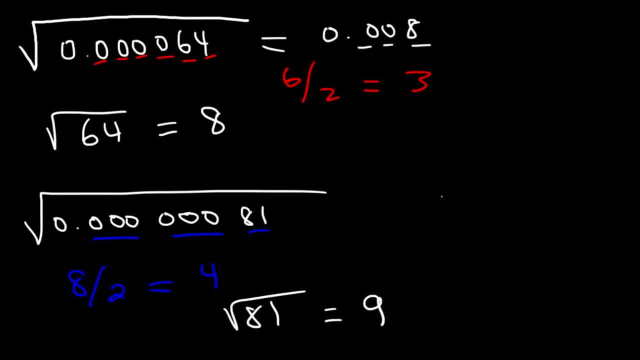 The square root of 81 is 9.. So to have 4 digits, we need 3 zeros and then a 9,. so 1,, 2,, 3, and here's a 9.. So that's the answer: .0009.. 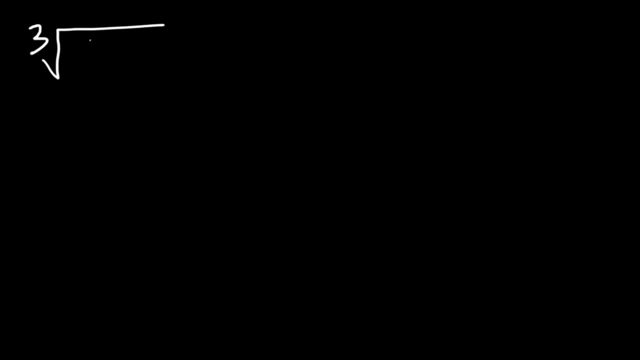 Now, what about cube roots? What is the cube root of .008?? What rules do we need to employ? Well, since the index number is a 3,, we're going to divide the digits by 3.. So, therefore, the number of digits has to be a multiple of 3.. 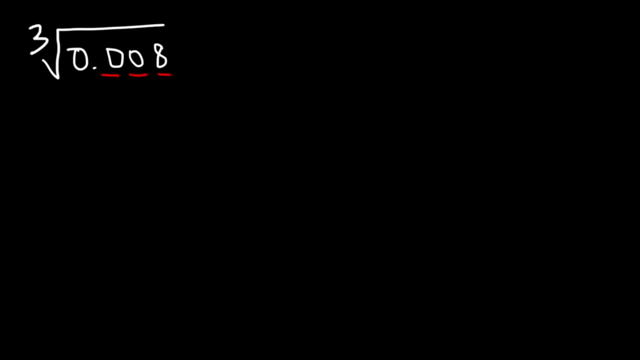 We need to get a whole number when we divide it for this to work. So here we have 3 digits. 3 divided by 3 is 1.. So the final answer should have only 1 digit, 1 digit to the right of the decimal point. 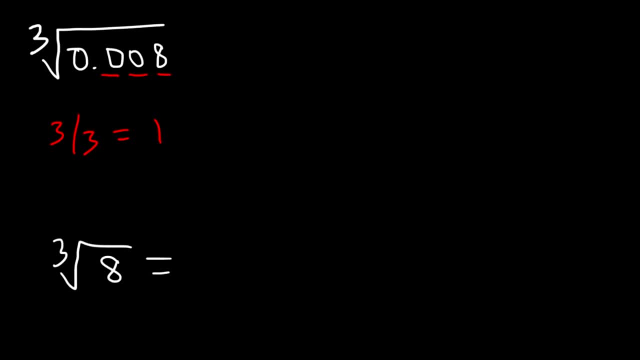 Now, what is the cube root of 8?? What number times itself 3 times is 8?. The cube root of 8 is 2, because 2 to the 3rd power is 8.. 2 times, 2 times 2, 3 times is 8.. 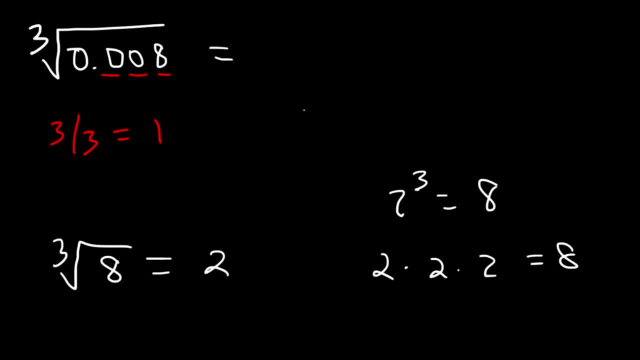 So if the cube root of 8 is 2, the cube root of .008 is going to be .2.. It's going to have 1 digit to the right of the decimal point. So, knowing that, try this example. What is the cube root of .000027??